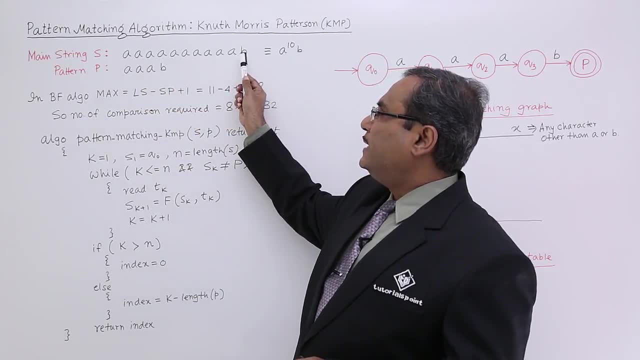 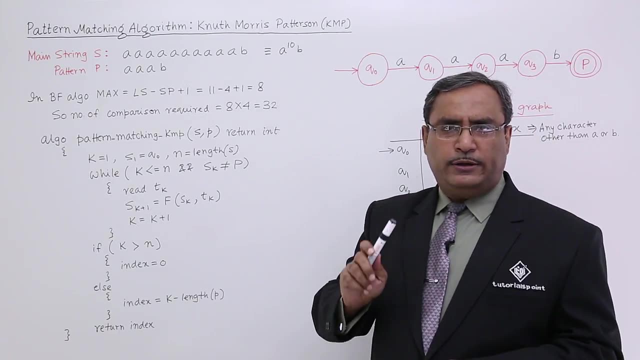 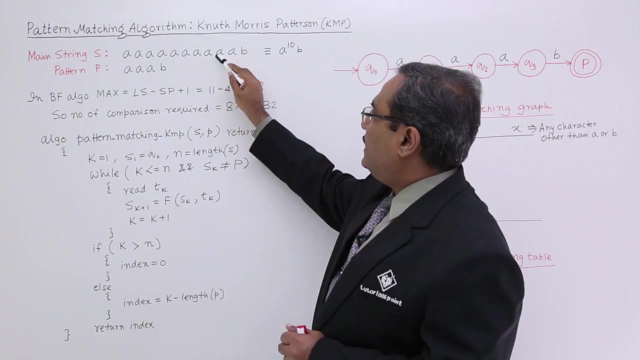 there is a main string which is having 10 times a and then b. So I am writing this one as a to the power of 10 b. Let us suppose the pattern which we are trying to search is a, a, a, b. Obviously I am getting this pattern here. This pattern is a, a, a, b. 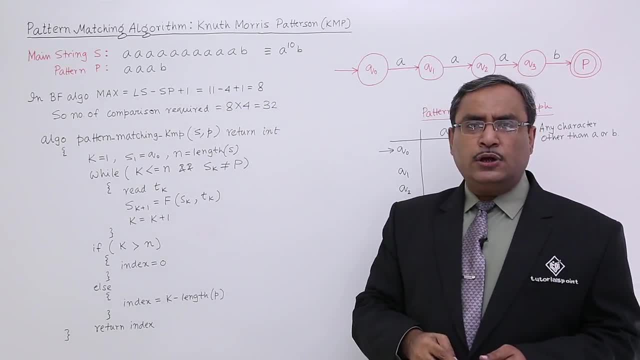 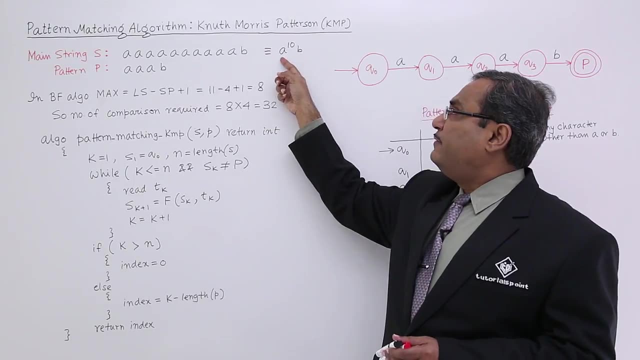 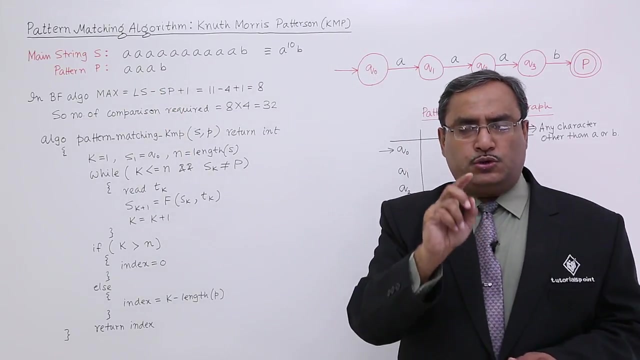 I am getting this one here. Okay, Now, in case of your brute force algorithm, what will happen? So here, this length of this main string is 11. So 10 times a and 1 times b, 11. And the pattern is having the length 4.. So how many times the pattern will get shifted? 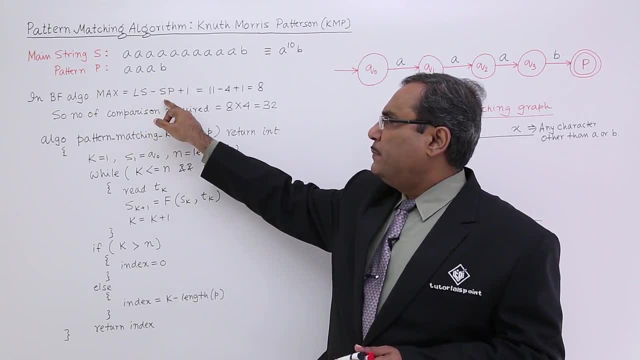 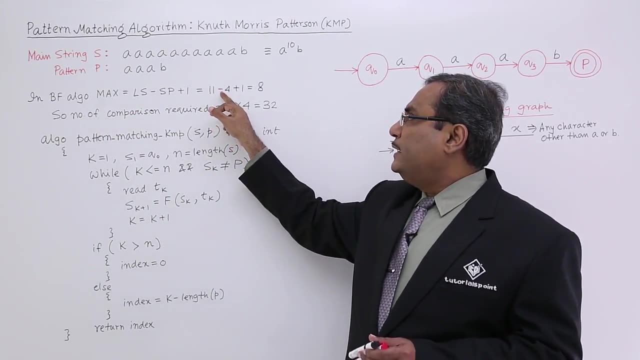 So that is length of the main string minus length of the pattern plus 1.. So that will be the max. Max number of times the pattern will get shifted will be 11 minus 4 plus 1. So 8 number of times. If you are not getting this one, please watch. 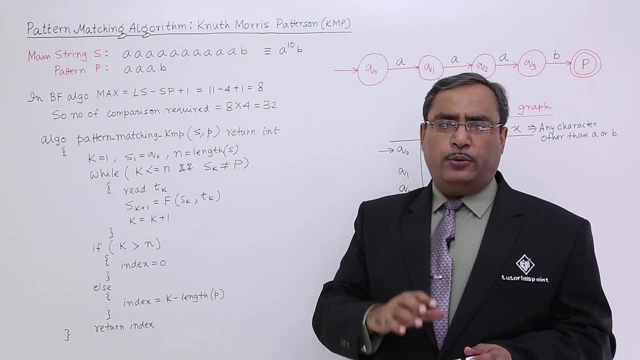 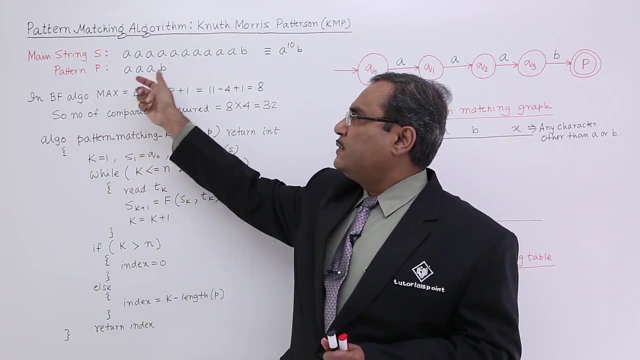 the previous video where we have discussed everything into the details with the algorithm, with the tracing example and all Okay. So in the brute force algorithm, the maximum times the pattern will get shifted for the matching will be 8.. Now think about the situation. 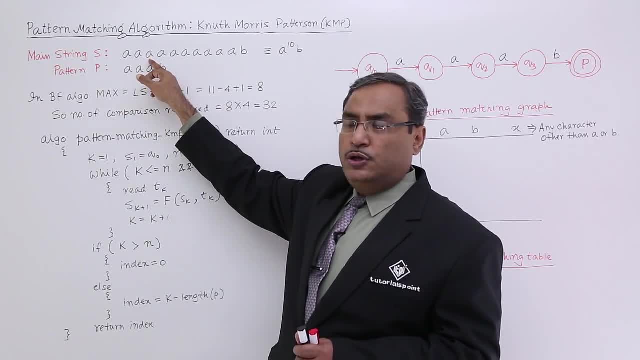 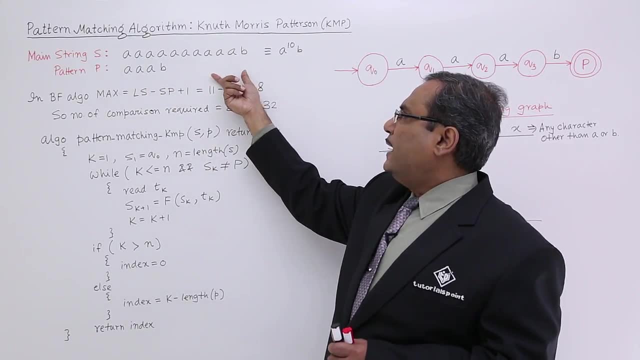 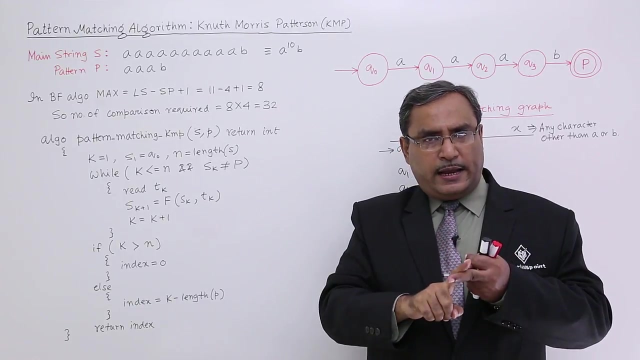 Each and every time the first three characters will match. So I shall go for the fourth character matching, and then I might be finding mismatch for all these cases, But at the last I shall get it. That means after placing the pattern under the main string. for each and every time I 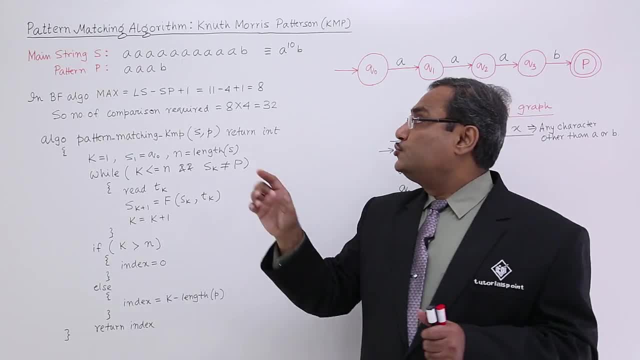 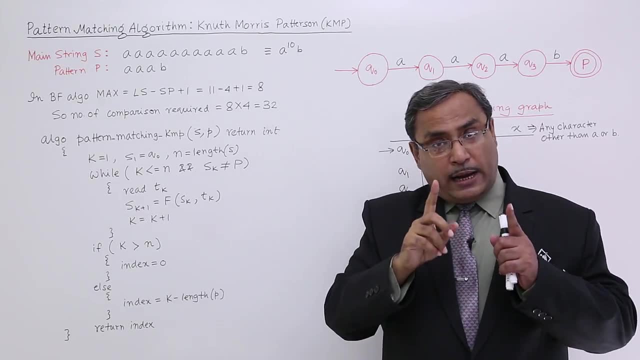 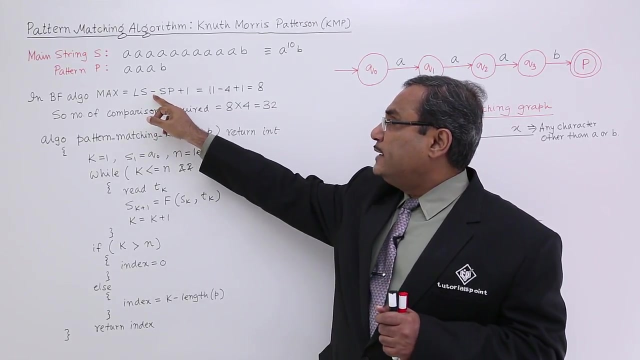 am going for 4 times comparison. So 8 times placing and 4 times comparison. So the total number of comparison required will be 32.. A question may come on this particular figure, also on this particular figure. So what is the figure? Figure is nothing but ls minus. 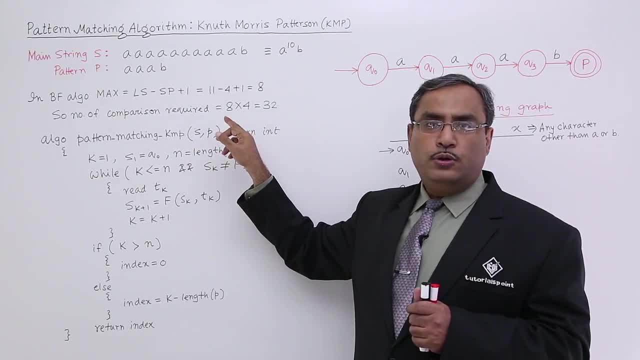 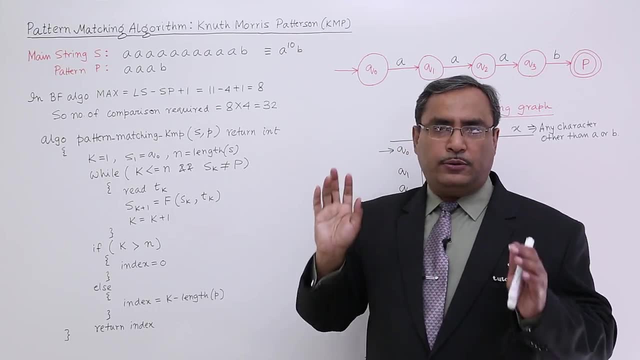 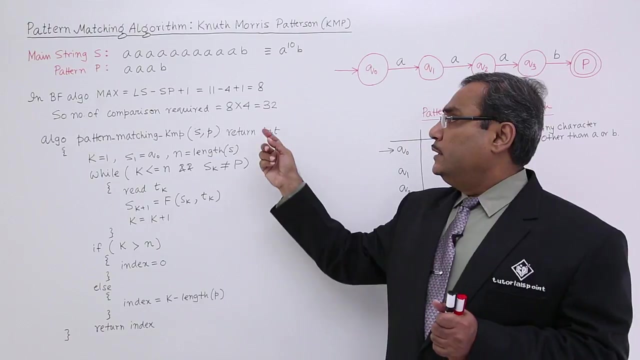 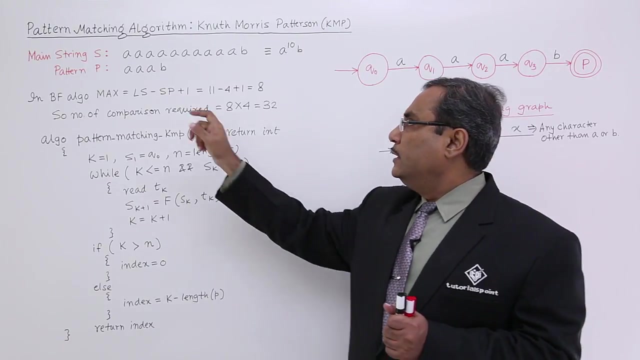 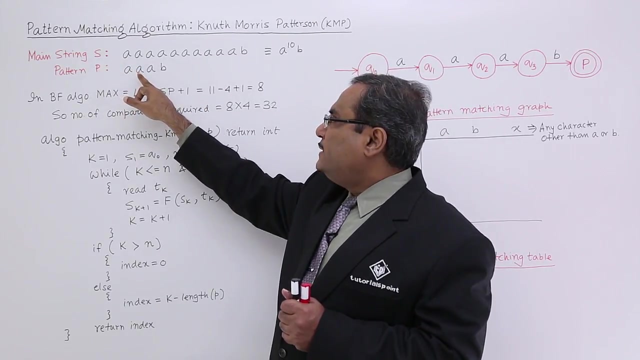 sp plus 1 whole into lp, whole into lp length of the pattern, The number of wizard�op matching Already. there is Steven here here, so this one be more or less the same. This one is more or less the same as this is the one that I had read earlier about. 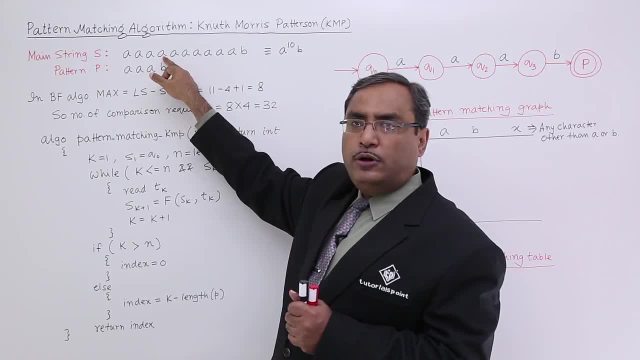 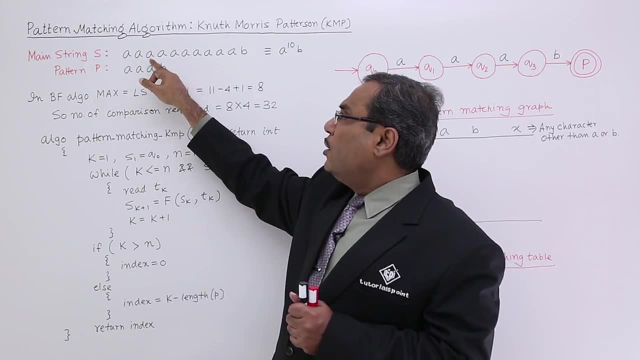 And so on and so forth. true, i'm matching b and a. i'm not getting. then why should i shift a pattern? and again, i shall have to check whether it is a or it is a or it is a already. i know that they are nothing but. 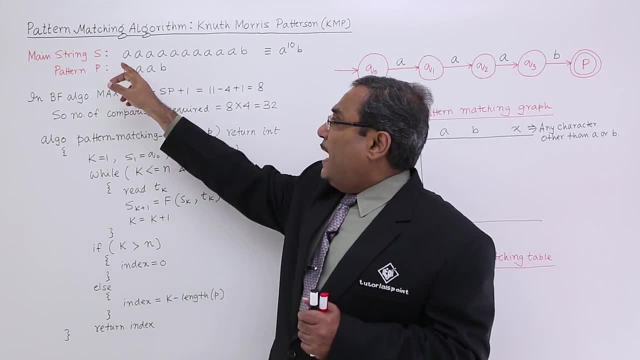 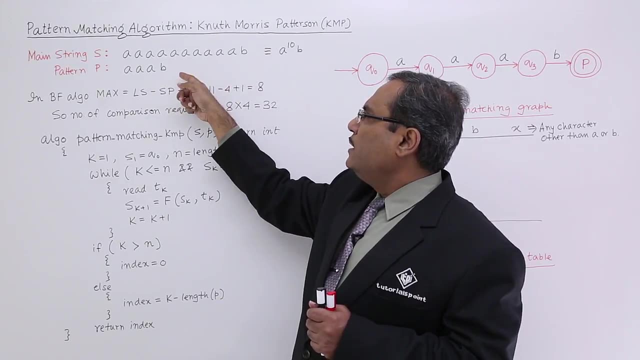 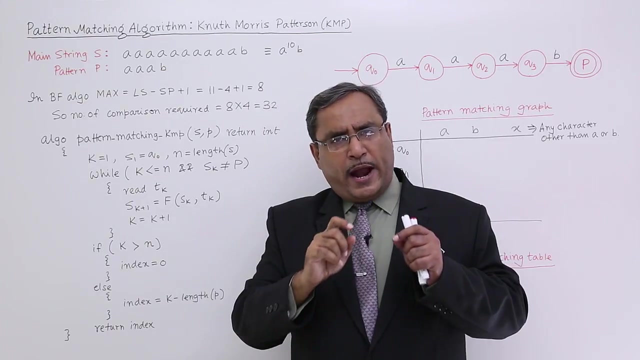 character a. then what should i do? as i'm getting a is there, so i shall wait for b, only b. i shall wait for only b. i need not to shift the pattern and go on checking whether it is a or a or a, because already i have checked i know the patterns are consisting of a's i required. 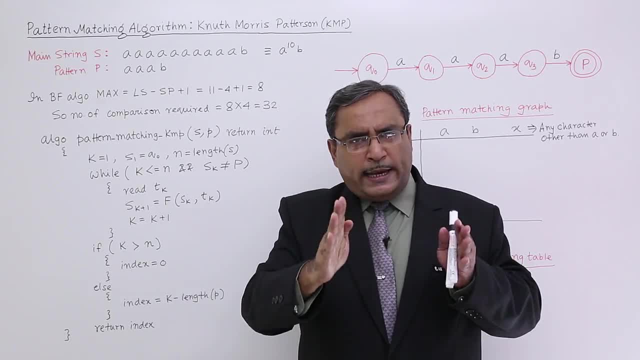 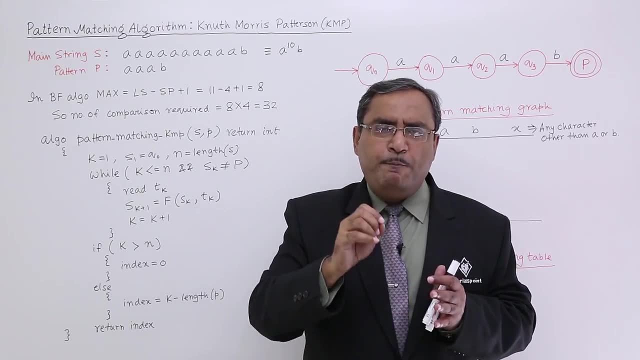 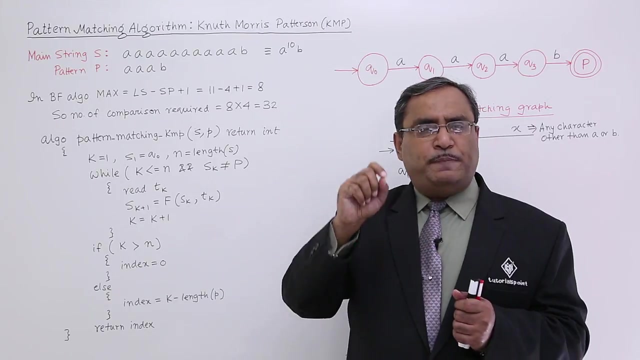 one b after three a's. so when i'm getting 10 times a, then obviously just i should skip, skip, skip until i get the b and then i shall announce that i have got the pattern. so in case of newt morris algorithm, newt morris patterson algorithm, kmp algorithm will be having how. 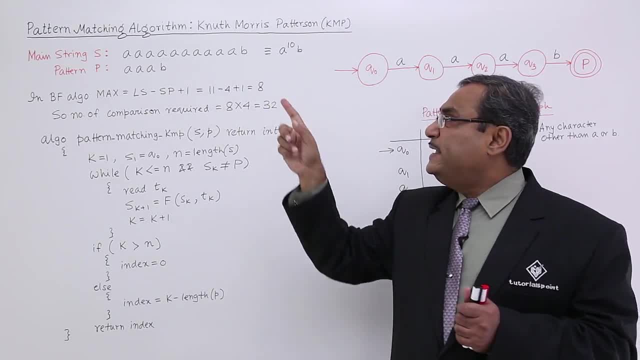 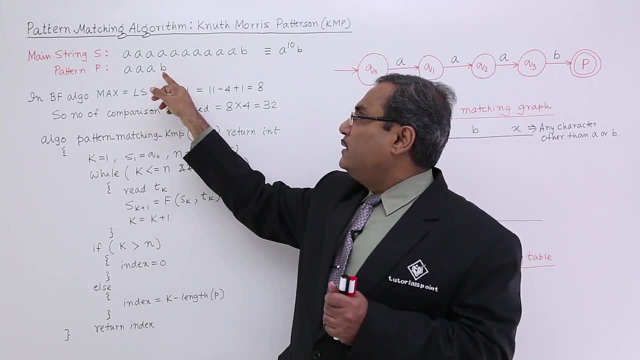 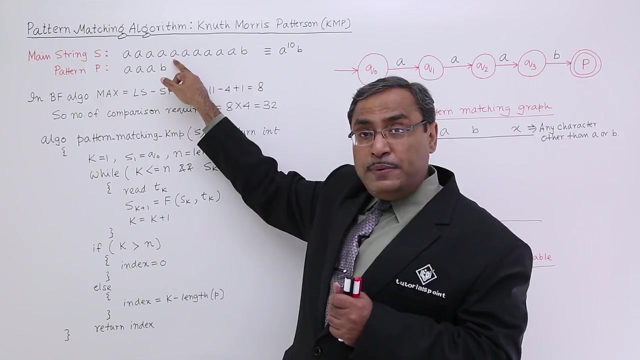 many times comparison. you, frankly speaking, will be having 11 times comparison, because i need not to go for comparison of a and a again and again when i shall get the mismatch that i'm finding a here, i'm finding b here. i know that four times a's are there. let, is it a b? no, it is another a. so i know. 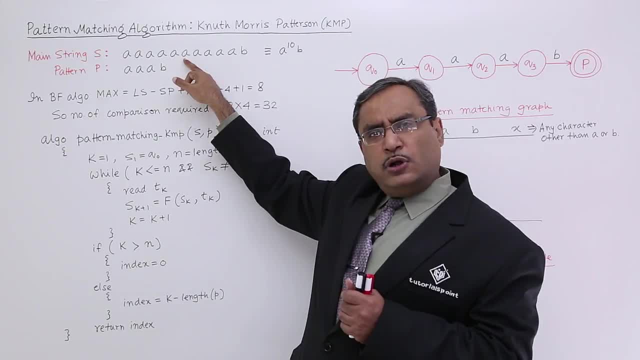 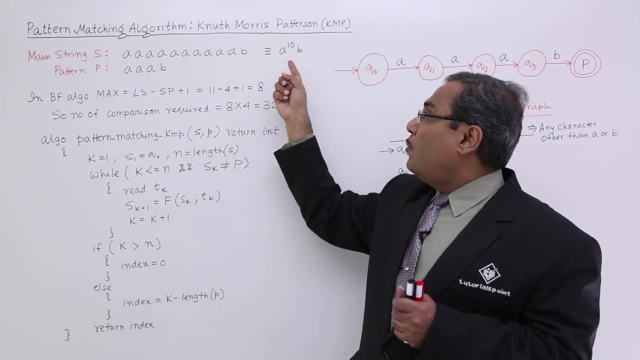 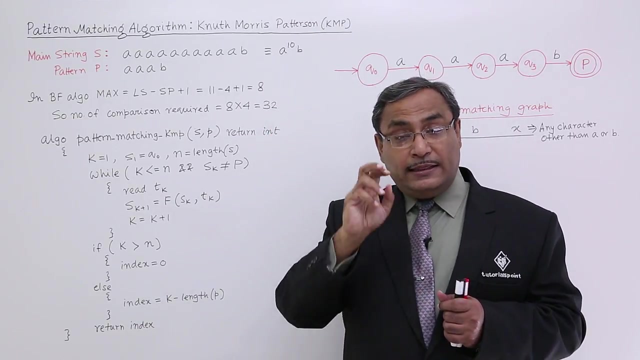 that three times a i have got. is it a b? it is also a. so i know that i have got three times a, is it a b? so in this way i shall go on doing so. how many times comparison will be required in kmp algorithm? instead of 32, i'll be requiring only 11 comparisons, and that is the main. 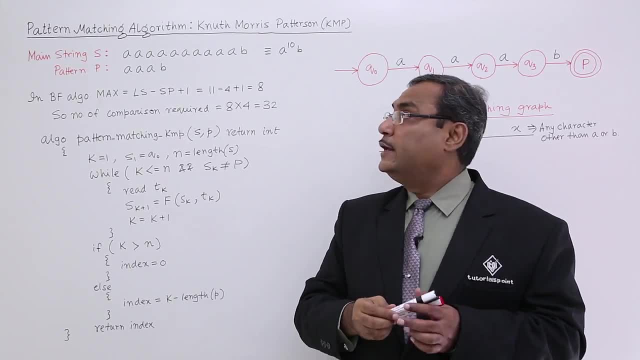 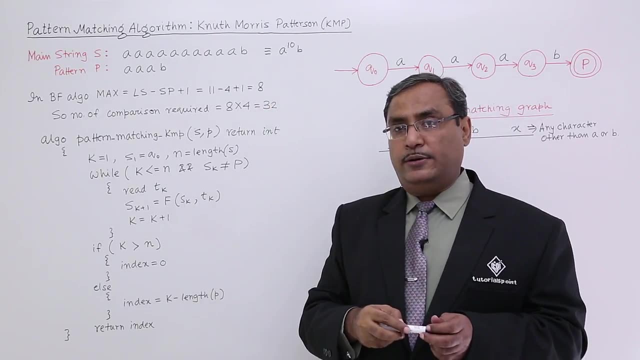 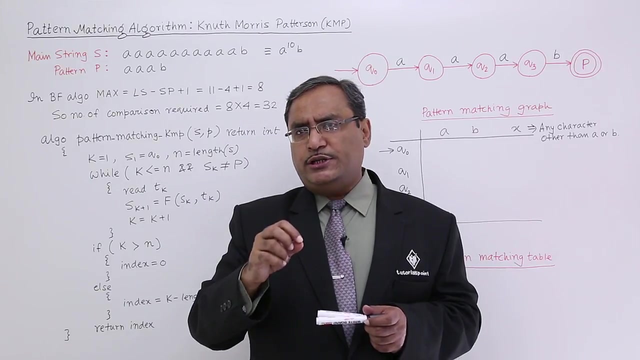 advantage of kmp algorithm. okay, so now i've got this idea why this kmp algorithm is better than this newt morris and patterson algorithm. so in the next video we shall go for the algorithm with the state transition table and state transition diagram to to guess the idea that how this particular 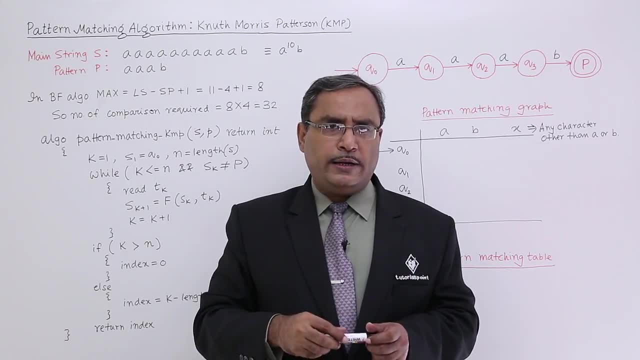 improvement in the pattern searching algorithm can be implemented. please watch the next video, and that will be in the continuation of this one. thanks for watching this one.